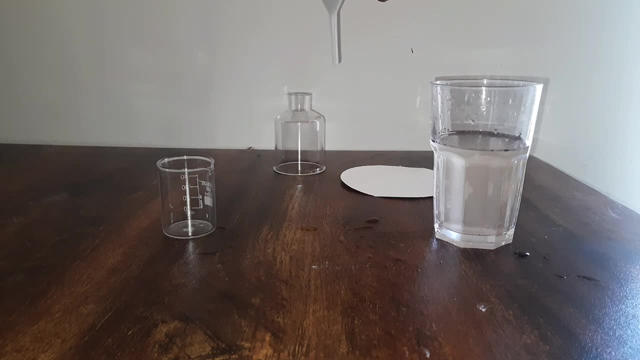 you can still use. you can still at least hold the funnel with your hand also, but it will take around five, seven minutes, or you can use a clamp stand. So, first step as a first step, what we will do is we will try and fold this filter paper and try and fit it into the mouth of this funnel. 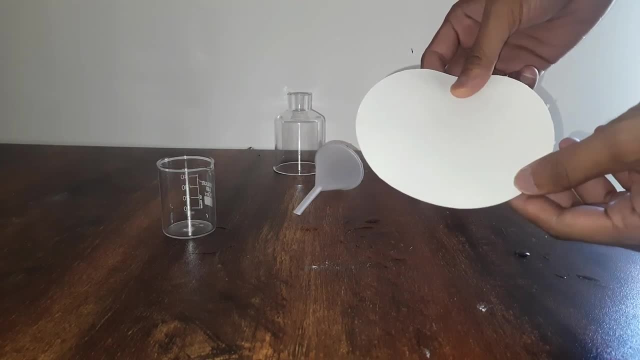 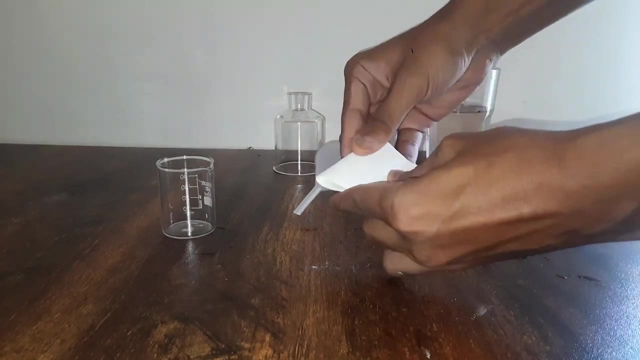 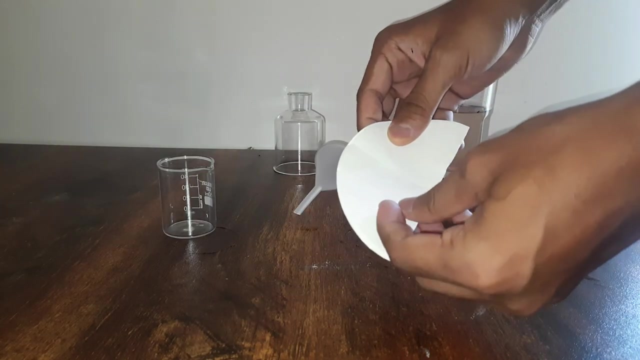 So to do that, we will first fold it in half, Then fold it in half again, Now try to open it, And once it is half opened, we hold this part inside and we try to put this part outside, just like this. 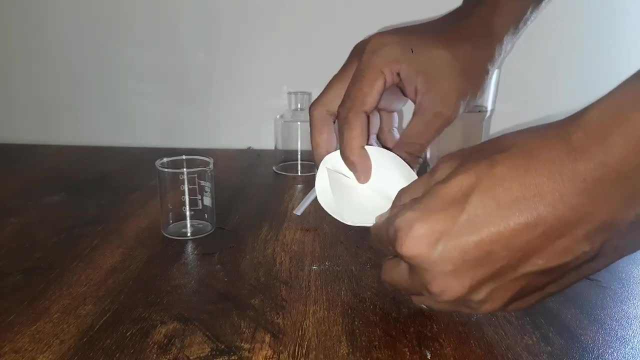 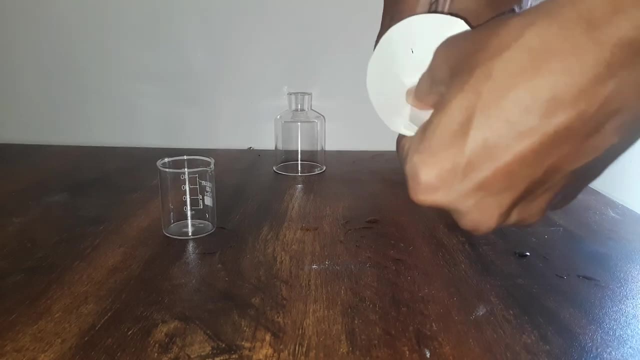 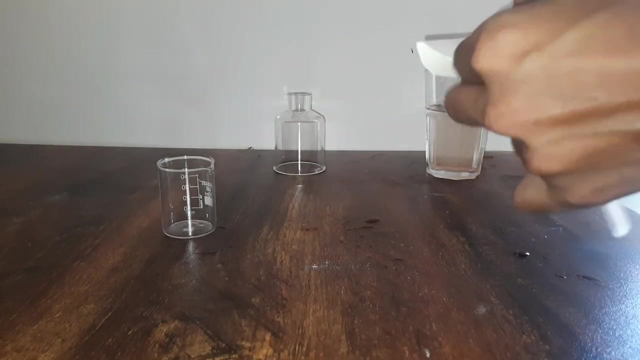 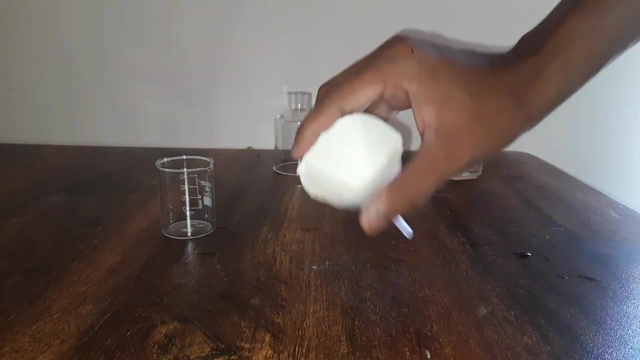 So so that a cone cone is formed, kind of like this, And then we can try and stretch it somewhat like this: Okay, next we try to fit this into the mouth of this funnel. All right, this is good enough. Next, what we'll do is we'll try to hold this funnel in place. 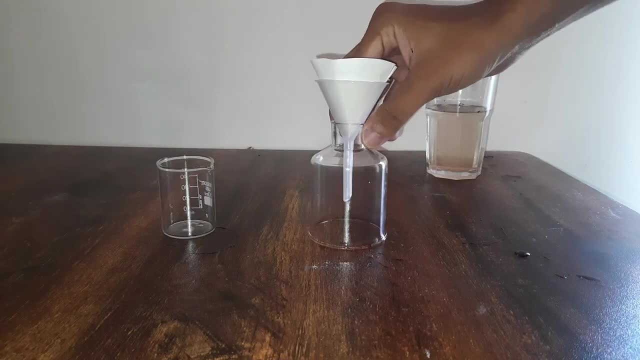 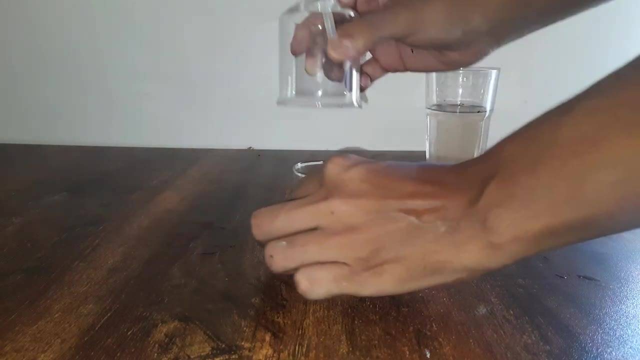 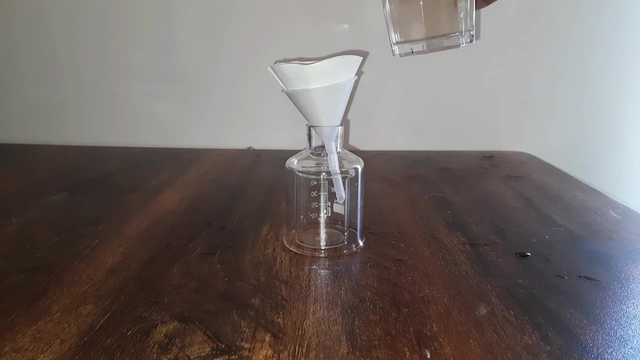 So I'm just gonna, I'm just gonna place it like this And keep an empty beaker below, below the other end of the funnel. Now I will pour this muddy water, this water with small sand particles dissolved, into this filter paper and wait for some time, and I want you to observe what happens. 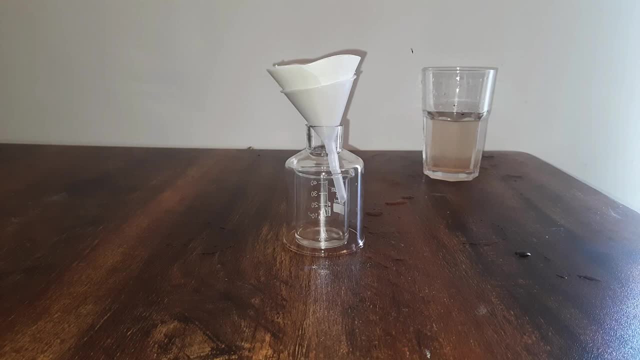 This process took around five to seven minutes. I have sped up the video so you are watching, watching it. go on, It should stop now. So now let's put it into the mouth. Okay, go by really fast, but it took around seven minutes. okay, we have enough collection in the beaker, let's. 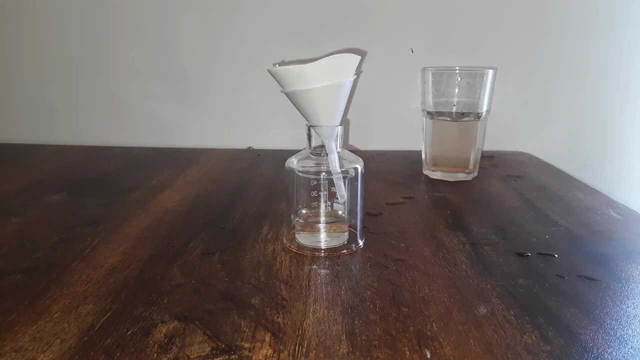 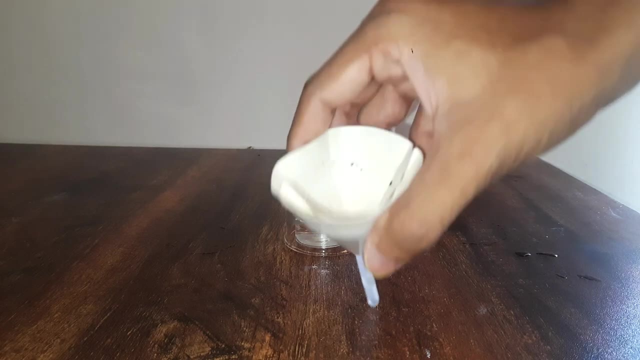 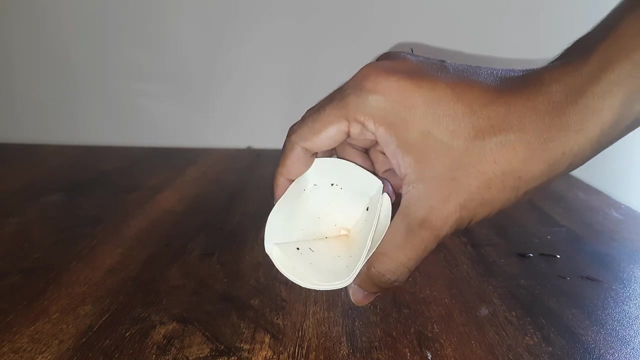 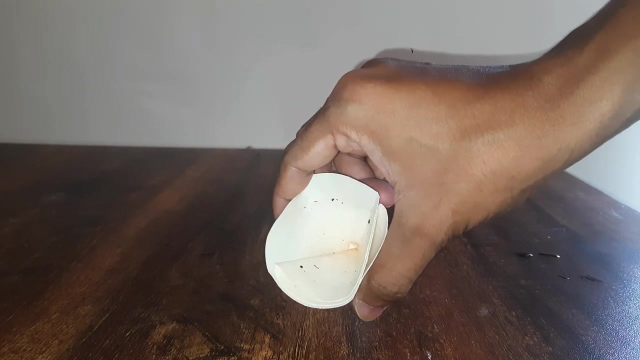 try to compare that with the glass over here. so we will remove, remove this funnel. have a look at all these sand particles that are filtered out. filter paper works great because they're extremely small holes in the filter paper which can allow the water to pass, but it can filter out the small sand particles. okay, let's.